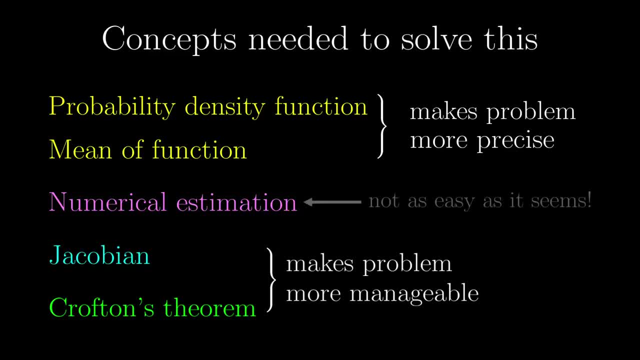 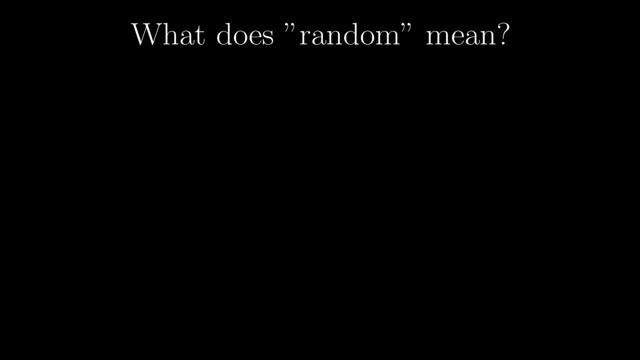 to estimating the answer numerically, because this is not as easy as it looks. To really understand the problem, we have to know what random means. The problem is a problem that can be solved by estimating the answer numerically. The problem can be solved by estimating the answer numerically. The problem can be solved by 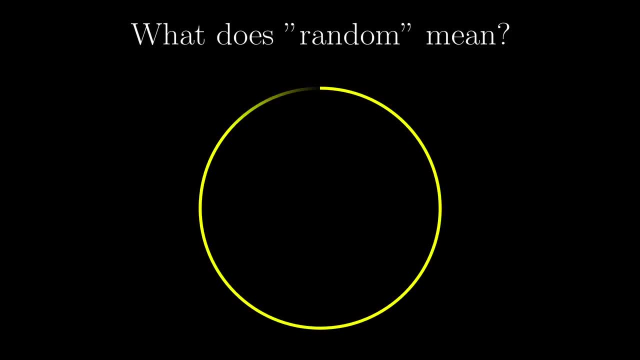 more precisely because we are picking pairs of points randomly for calculating distances. Ideally, what we want is that our points are roughly uniformly distributed. This means that if there are 4 points in this box, if I move the box elsewhere, it should contain more or less. 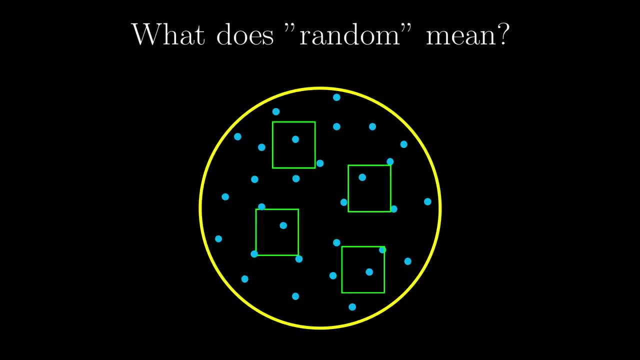 4 points as well. The areas of the boxes can vary, but the number of points in these boxes should be more or less the same. In other words, the density of the points should be the same across the disc. However, the density of points depends on the number of samples taken. 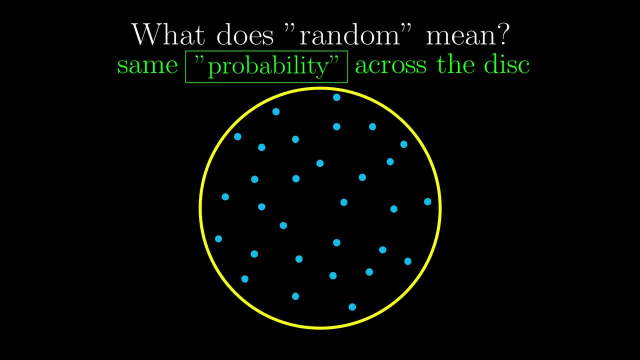 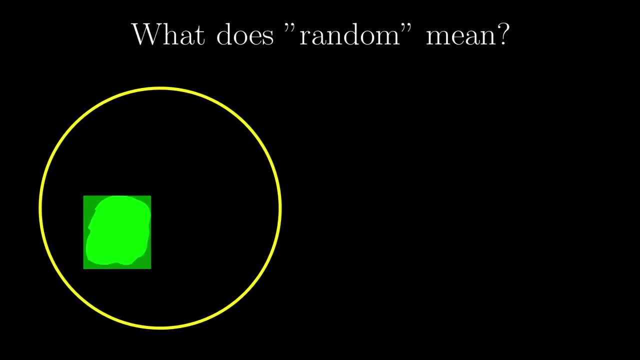 so a better description would be having the same probability across the disc. This means that the probability of any point being in this box will be the same as that in any other box, as long as they have the same area. The box does not have to be rectangular, and any shape would. 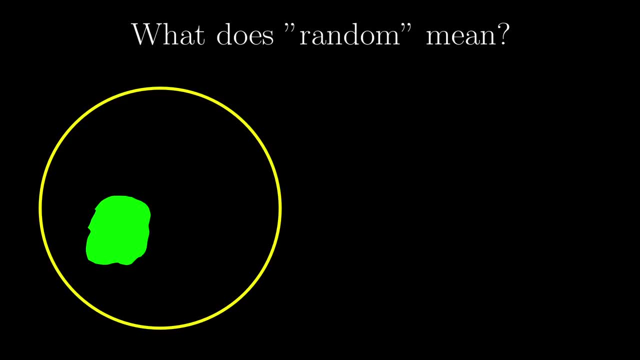 be the same. The box does not have to be rectangular and any shape would be the same, be fine, but rectangles are just easier to demonstrate. Anyway, the probability of a point inside a region would be proportional to the area, In other words, the ratio between 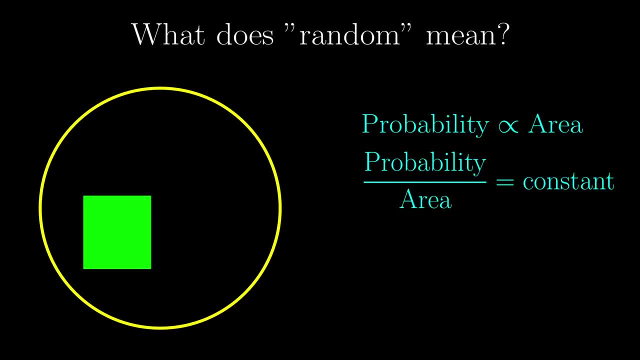 probability and area of the region is a constant. This quantity on the left is probability density. so actually we were not thinking about probability at any given point. when we say same probability across the disc, We actually meant probability density. We can actually calculate this constant of probability density When the 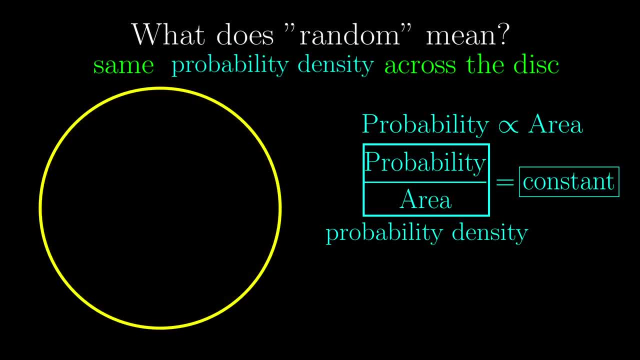 area concerned is the entire circle, ie the area being pi, the probability is, of course, 1.. However, in other cases, this quantity can depend on position ie, a function of the position vector x. This function is unsurprisingly called probability density function- pdf for short, The 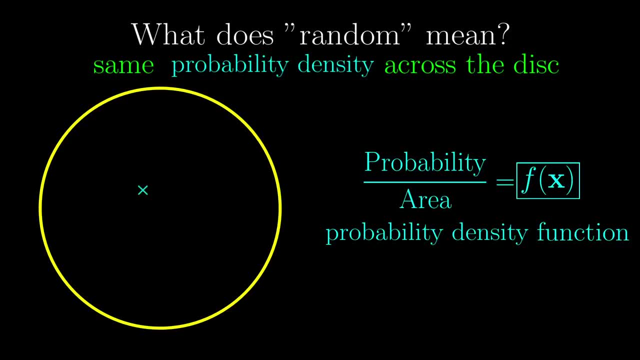 way to calculate the probability density function is to use the probability density function function to calculate the probability density at one single point works like this: Pick any region around the point and calculate the ratio between probability and area of the region. If we shrink it, this ratio might change a little bit. The pdf at this point is taken. 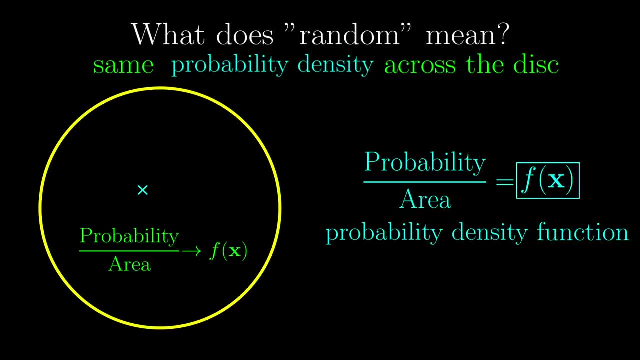 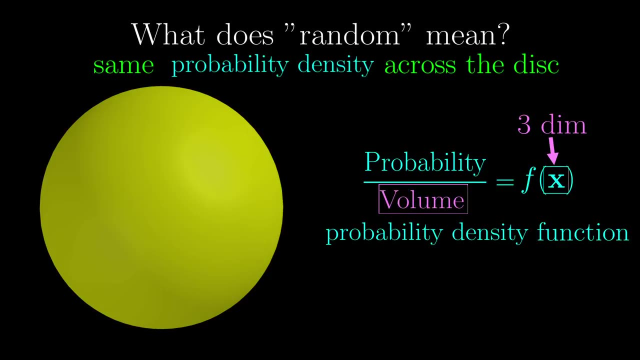 to be the limit of this ratio when the region shrinks to nothing. In this case, the position vector is in two dimensions, and so the denominator is naturally the area of the region. If we are working in three dimensions, the denominator would be the volume instead, and so on. 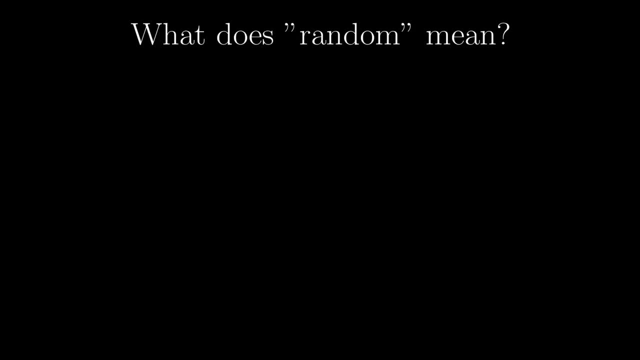 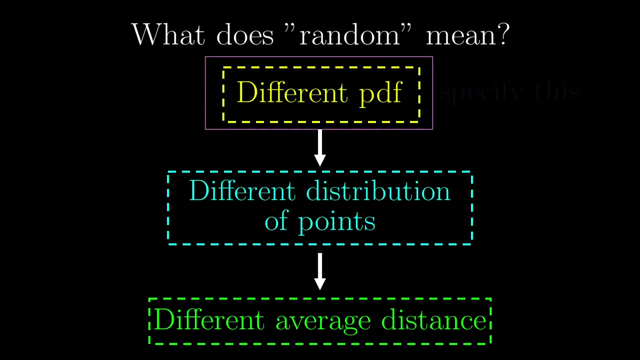 It might seem like the discussion of pdfs is irrelevant, but if we have different probability density functions then we will have a very different distribution of points and thus different answers to a problem of average distance. In general, whenever you say random, you should always specify the pdf to avoid getting different answers to the same. 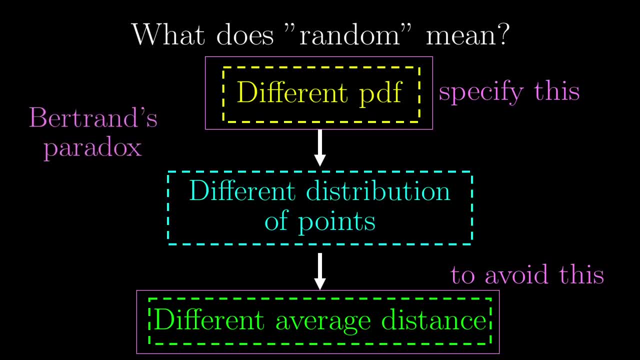 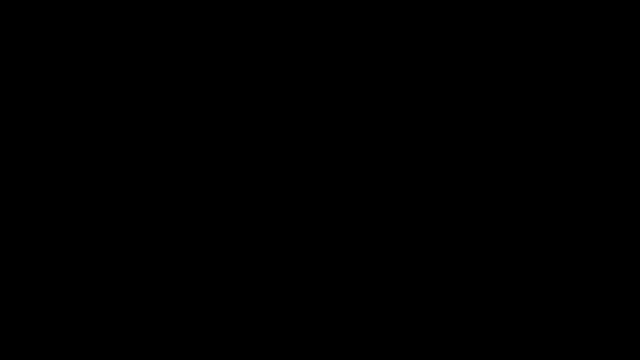 So let's start with the first question. This is basically the crux of the infamous Bertrand's paradox, which might be a story for another time. Anyway, the next thing we need to deal with is the word average, because there is a continuum of possible distances and pairs of points. 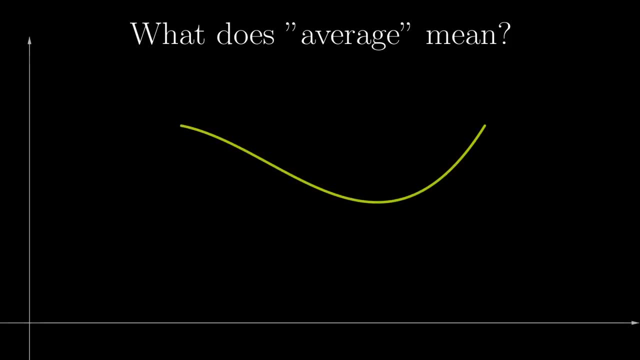 But let's deal with the simpler situation first. What would be the average of a function like this? Intuitively, we should sample some values of the function and then we can calculate the average of the function. For example, if we were to use the 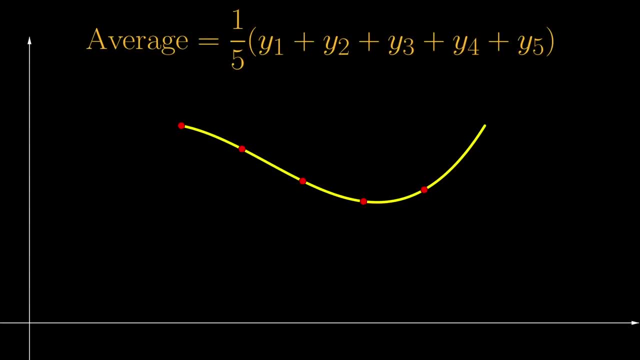 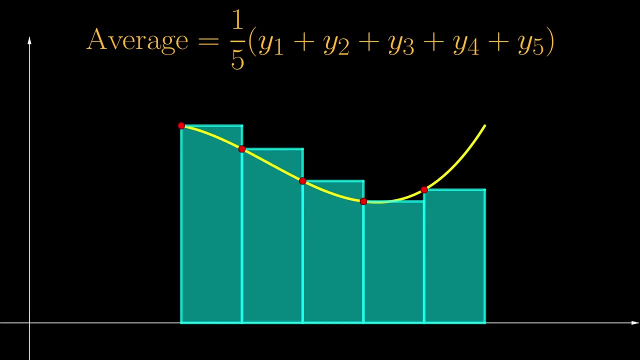 y-coordinates as y1 to y5, then our estimate of the average would be summing them up, then divide by 5.. On the other hand, we can consider the area of these rectangular strips. We chose the points at regular intervals, so the area of the strips is the common width times the sum of the y's. 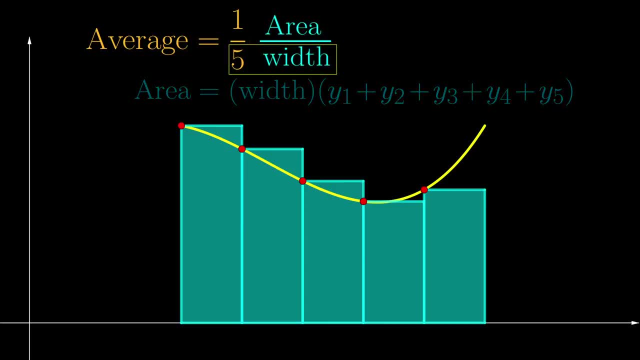 With that we can replace the sum by area over the common width. However, we don't know precisely the length of the interval on which the function is defined. so if the function is defined on the interval, then the 5 times width here can be replaced by. 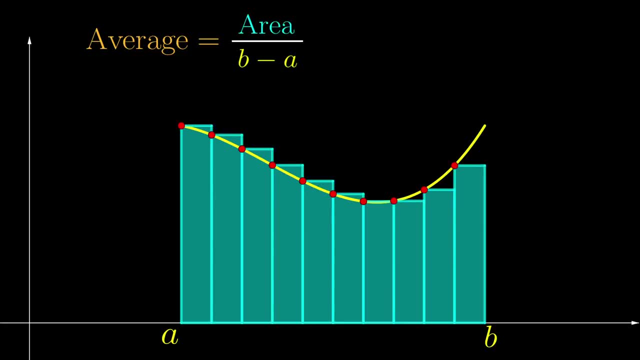 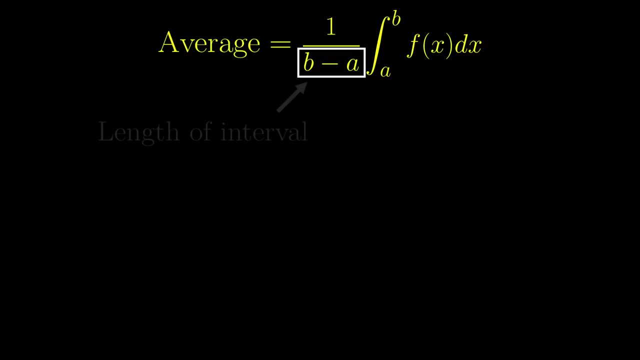 b minus a. If we sample more points, then the area of the rectangular strips becomes closer and closer to the area under the curve. so the average can be found with an integral. Now notice that the denominator is the length of the interval And we are integrating over the interval If the function takes in higher dimensional input. 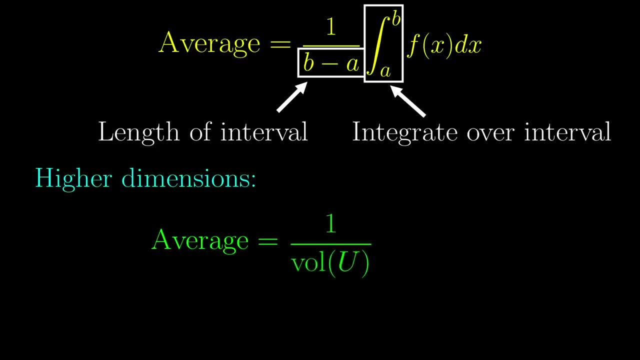 then the length of the interval would be generalised to the volume of the domain And instead of integrating over an interval, we integrate the function over the domain. In fact, the pre-factor is the probability density across the domain. so if the PDF is not constant, this average will be more complicated. Anyway, to determine the 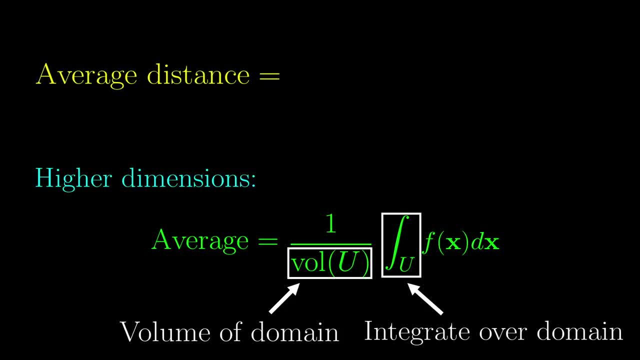 average distance. we need to first determine the domain of the function. Here the function would be the distance between the points x and y. X is a point in a unit disk centred at the origin and of course y is also a point in the unit disk. That means 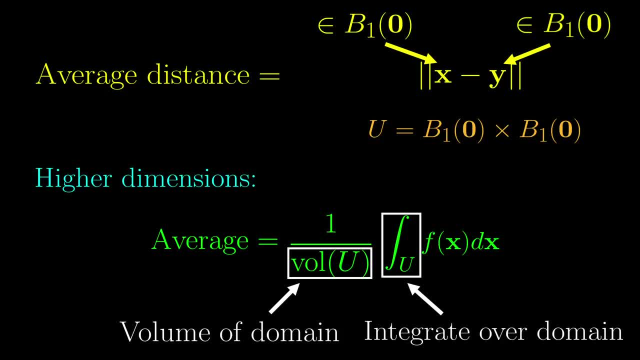 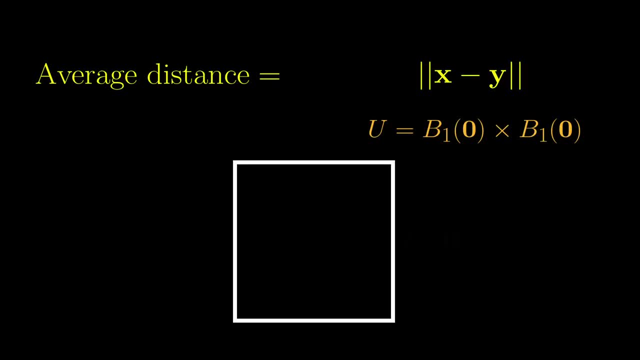 the domain is the ordered pairs of points in a unit disk. Even though this is a 4-dimensional domain, it is useful to think of it as a sort of square where each side represents a unit disk. So calculating the 4-dimensional volume of the domain u is sort of like calculating 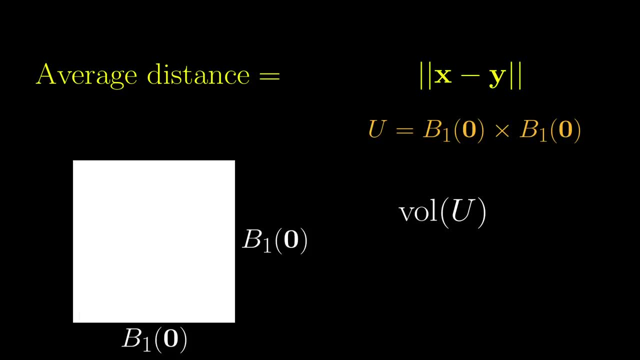 the area of a square It would be side length squared. but here we generalise the side length to be the 2-dimensional volume or the area of the unit disk. Area of a unit disk is pi, so the volume of the domain is pi squared. So, going back to the formula for the average, 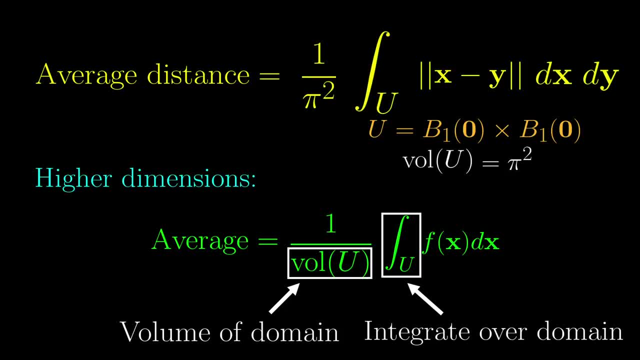 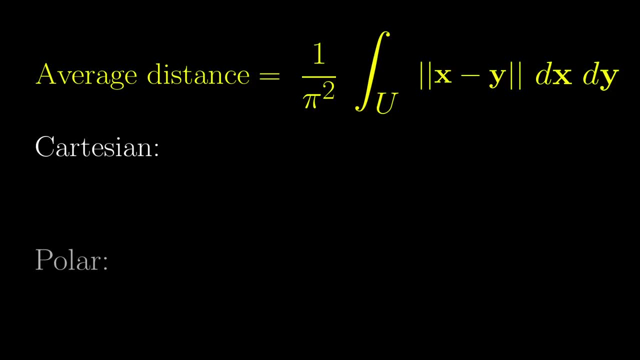 of a function. we can simply substitute the domain and the volume To make this integral more explicit. we can choose to represent the points in Cartesian or polar coordinates. However, whichever coordinate system you choose, the resulting quadruple integral is really really horrible. If we don't know the answer, there is no reason. 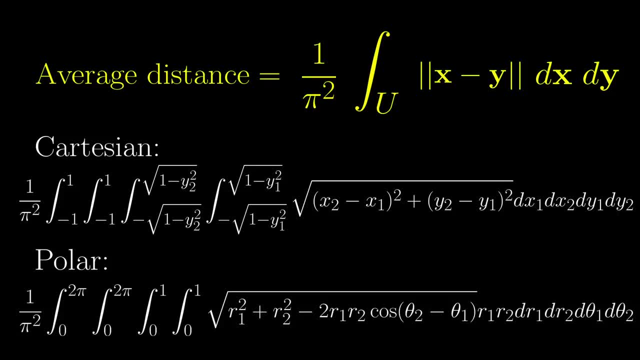 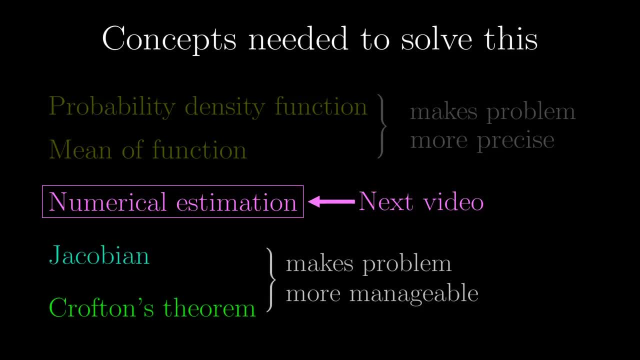 why this evaluates to a nice closed-form answer, which is why in the next video, we want to numerically estimate the answer first. Then the following videos will explain the remaining two concepts that allow us to solve this problem analytically, which will be in next year. 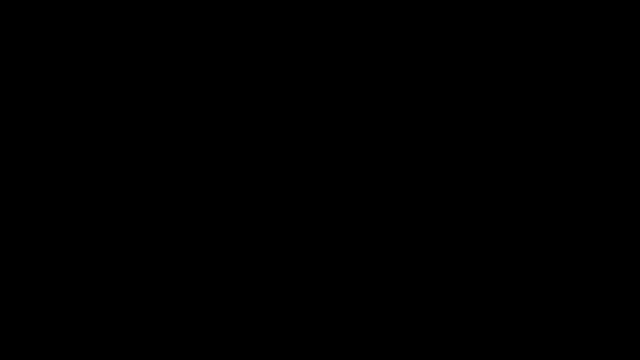 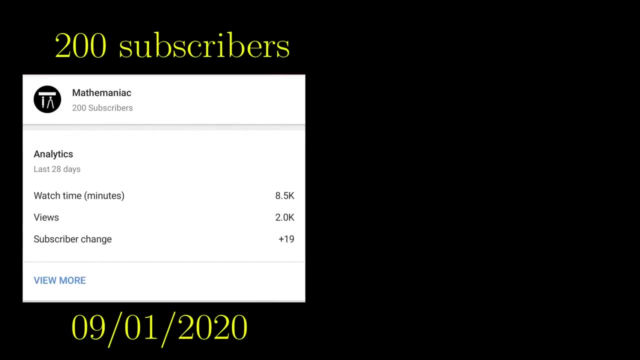 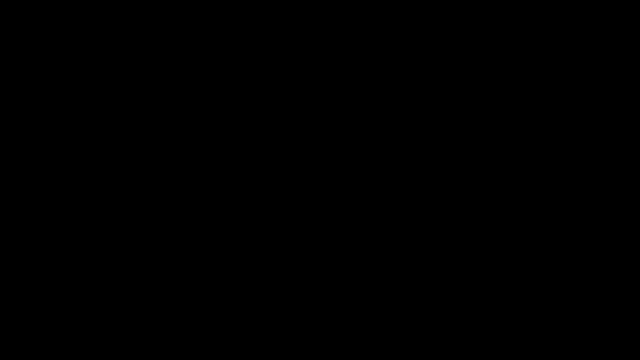 because this will be the last video in 2020 from me, so I would like to give a big thanks to all of you. In the beginning of this year, I only had 200 subscribers and, as of recording, I have more than 2000 subscribers. Merry Christmas, or if you don't celebrate Christmas,